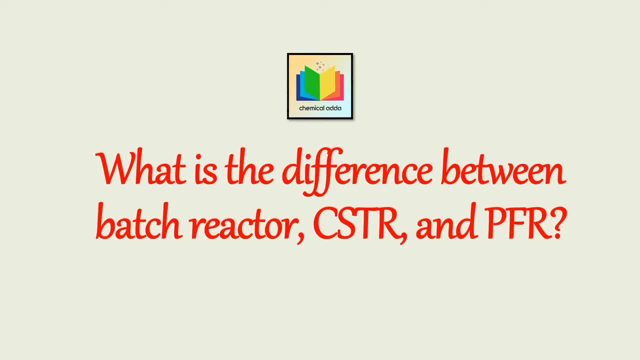 so chemical reactors vary widely in size, shape and in the method of operation. but there are three basic reactors used in the chemical industry, which are: batch reactor, continuous stirred tank reactor, that is cstr, and plug flow reactor, that is pfr. so let's see the difference between these three basic reactors. 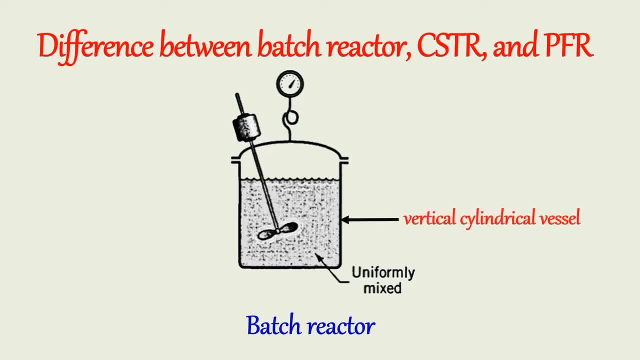 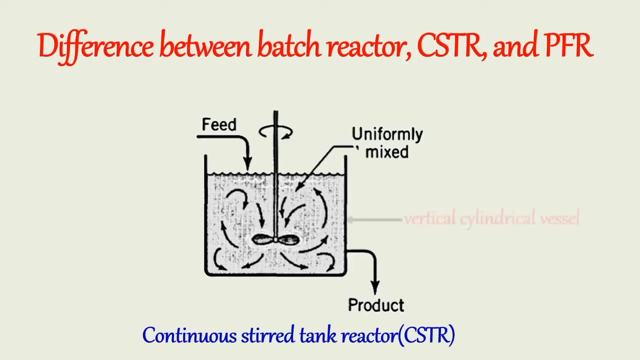 so batch reactor consists of a vertical cylindrical vessel equipped with an agitator or stirrer for stirring the contents. it is also provided with either an external jacket or cooling coil, or both, for heating or cooling the reactor contents. cstr, that is, a continuous stirred tank reactor, is a vertical cylindrical vessel equipped with. 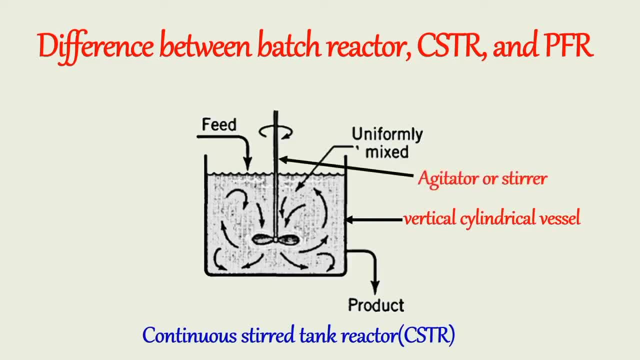 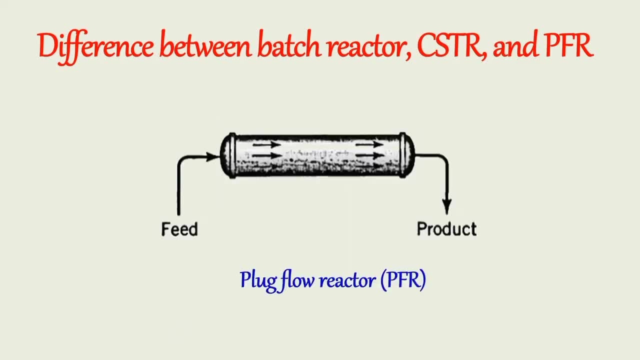 a mechanical stirrer and provision for heat transfer. cstr is also called a back mix or mixed flow reactor. pfr, that is, plug flow reactor, is a single continuous long tube or several tubes arranged parallel. it is also provided with either jacket or shell and tube type design for heat. 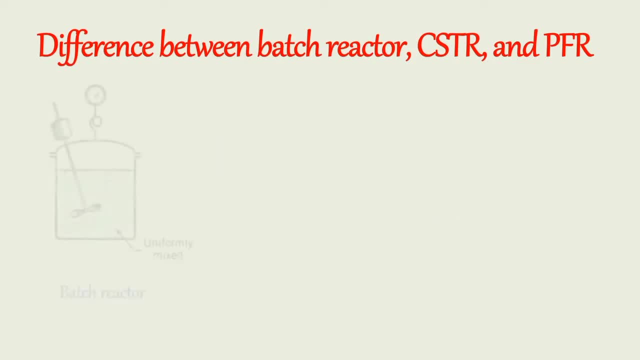 transfer then in a batch reactor. the reactants are charged at the beginning into a container, left to react for a certain period in the reactor under certain agitation, during which no material is fed or removed from it, and the resultant product mixture is withdrawn at a subsequent time. 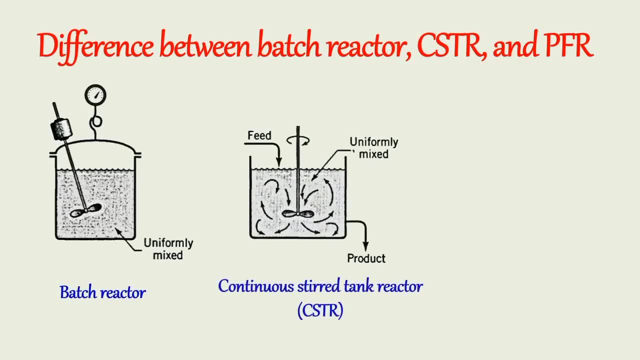 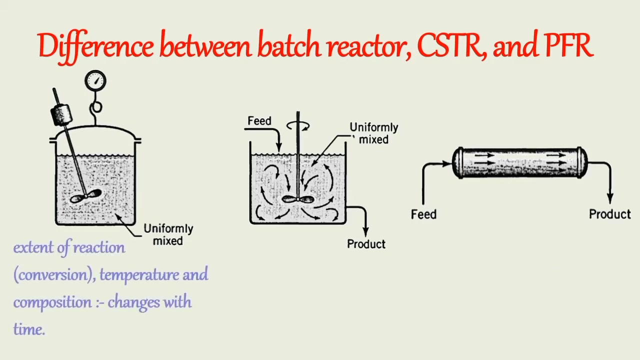 in cstr reactor, reactants are introduced and the product mixture is withdrawn simultaneously in a continuous manner, due to which certain pool of reaction mixture is always maintained in it. in pfr, reactants enter at one end and the product mixture leaves from the other end in batch reactor the extent of reaction, that is, conversion. 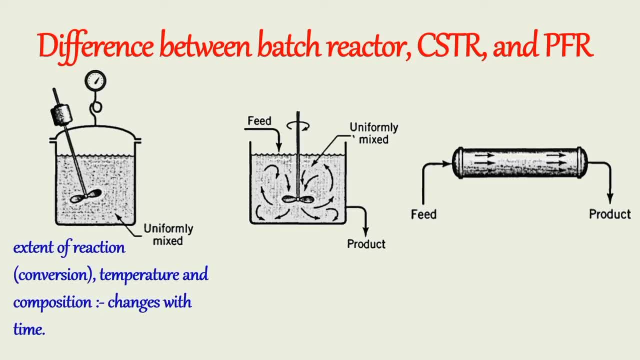 and properties such as temperature and composition changes with time, but at any instant of time the composition is uniform throughout the reactor zone. in cstr, contents are well stirred so that the properties of reaction mass, such as temperature and composition, are uniform throughout and hence the exit stream from the. 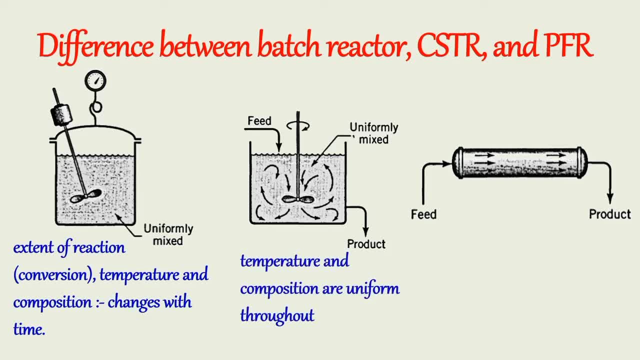 reactor has the same composition as the fluid within the reactor. in pfr there is no mixing in the direction of the flow and there is complete mixing in the radial direction, you hence in the axial direction, the elements of fluid of the reaction mass independent of each other. that means each one has different composition and 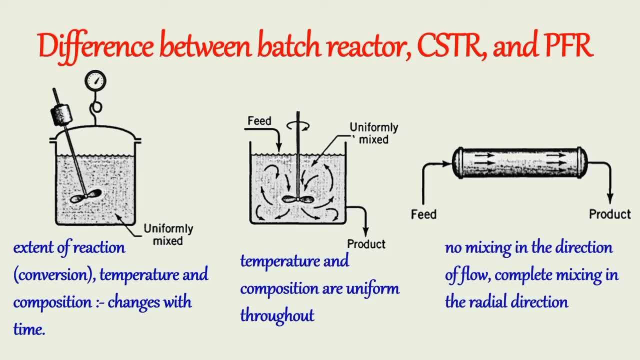 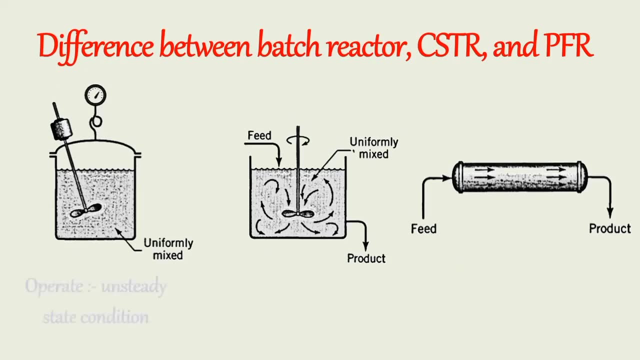 temperature, and such type of flow pattern is called plug flow. therefore, in a plug flow reactor the extent of reaction, temperature and composition may vary with the position in the reactor. the batch reactor operates under unsteady state conditions, but cstr and pfr normally run at a steady state. 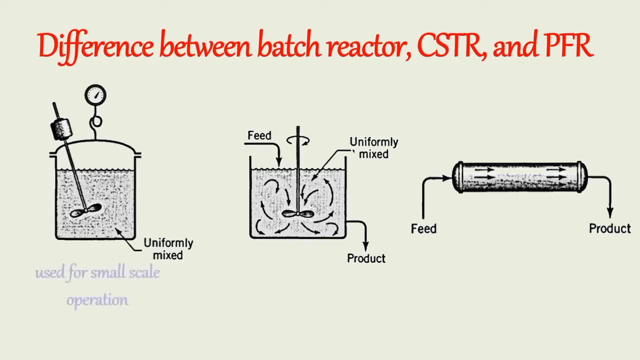 a batch reactor is used small scale operation, but cstr and pfr can be used for large scale operation. then batch reactor and cstr are used for liquid phase reactions and pfr is mostly used for gas phase reactions. a batch reactor is used for liquid phase reactions and pfr is mostly used for gas phase reactions. 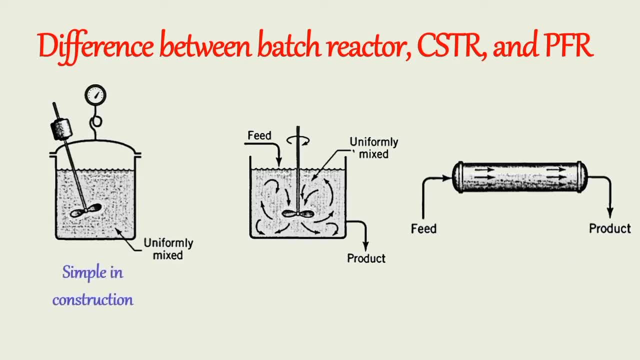 a batch reactor is used for liquid phase reactions and pfr is mostly used for gas phase reactions, then batch reactor certainly operates in Solo supervised production. a batch reactor is used for use in single stage blast research. the batch reactor is essential for the other structures. the batch reactor is applied by Metroid alloy. 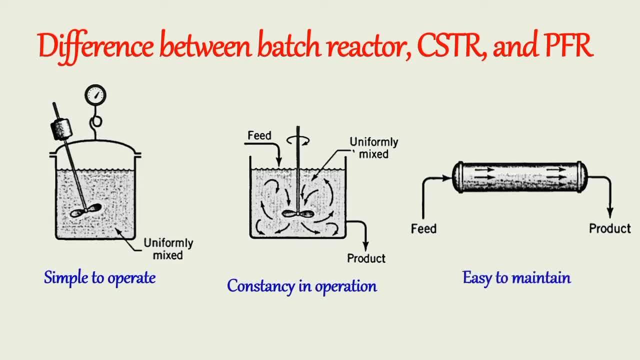 in the surface of the reactor. the batch reactor is simply in construction. it has the flexibility of operation. cstr offers greater constancy in operating conditions and hence offer greater constancy in the quality of the products. pfrs are relatively easy to maintain as there is no f 이야기. they can be fearsome for available high quality applications. 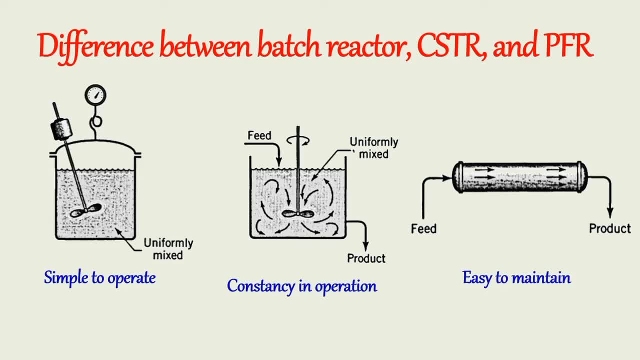 as there is no f מע activity in operations, is no moving parts in a batch reactor. high conversion can be obtained by leaving the reactant in the reactor for long periods, but the disadvantage is it required high labor cost per batch, then variability of products from batch to batch and the difficulty of large scale production. 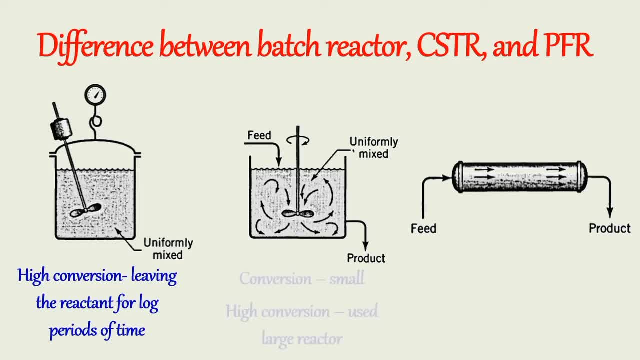 then in CSTR, conversion of reactant per unit volume of the reactor is small, hence to obtain a high conversion, consequently very large reactors are required in a plug flow reactor. the highest conversion per unit volume of the reactor can be obtained in the batch reactor. the initial cost is quite low and the operating 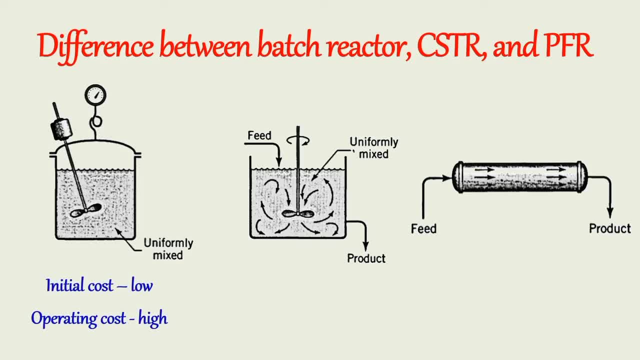 conversion of reactants per unit volume of the reactor can be obtained. if the temperature is. cost is high In CSTR and PFR initial cost is quite high And the operating cost is low. CSTR and PFR required little supervision And well suited for automatic control. The batch reactor can be used. 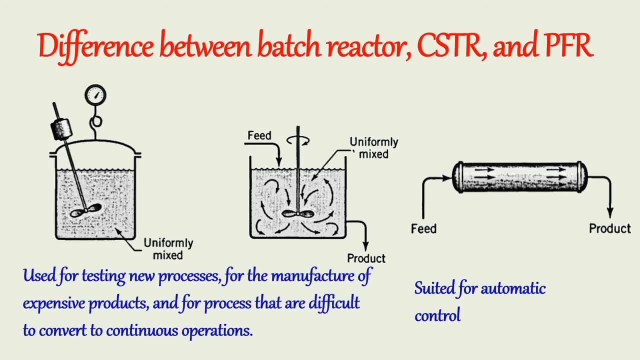 For testing new processes that have not been fully developed, For the manufacture of expensive products And for processes that are difficult to convert to continuous operations. CSTR can be operated under isothermal condition Even when the heat of the reaction is high In a plug flow reactor. 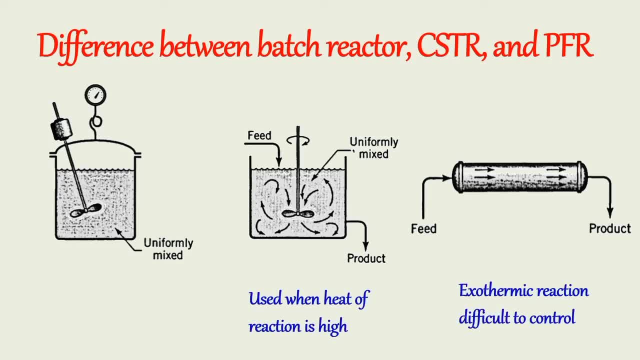 For exothermic reactions It is difficult to control the temperature And hot spots can occur. CSTR cannot be used for High pressure reactions Because it requires a large wall thickness And complex sealing arrangements for agitator, Which increases initial and maintenance cost. 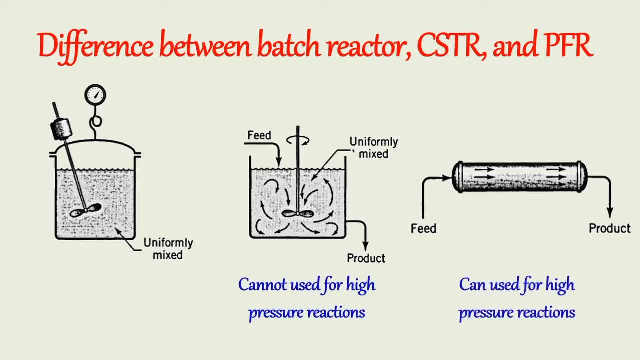 PFR can be used for high pressure reactions because of cost considerations. As it uses small diameter tubes, CSTR is not suited for reactions with a very high heat of reaction Due to low temperature. CSTR can be used for high pressure reactions Because it requires a large wall thickness. 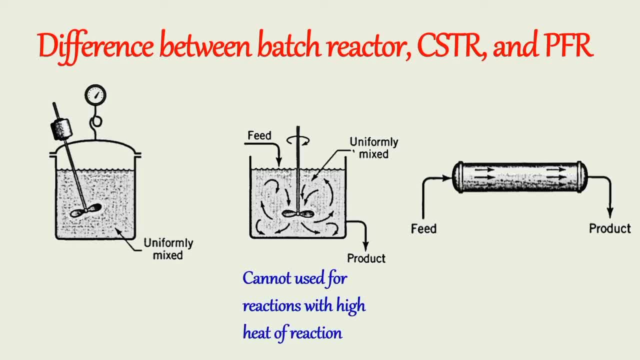 And low area heat transfer is available per unit volume And low heat transfer coefficients. PFR can also be used for reactions with the high heat of reaction, As the rate of heat transfer per unit volume of the reaction mixture is high. For batch reactor mole balance equation in differential form is: